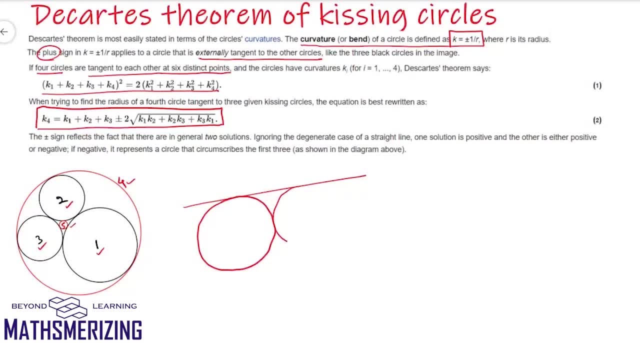 Suppose I have to find a circle which touches the straight line and the two given circles, then also I can use Descartes theorem for kissing circles. For a straight line we assume that radius of the circle is infinite and for that the value of k will be zero. So, assuming k to be zero, we 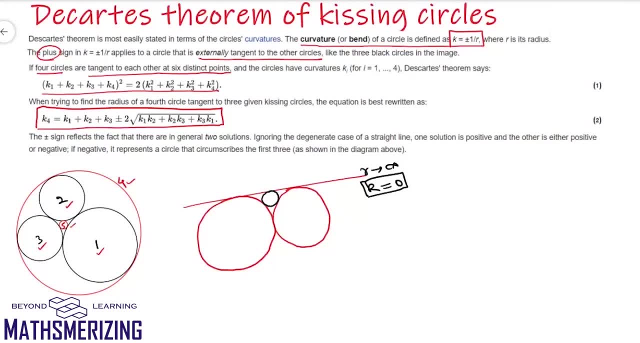 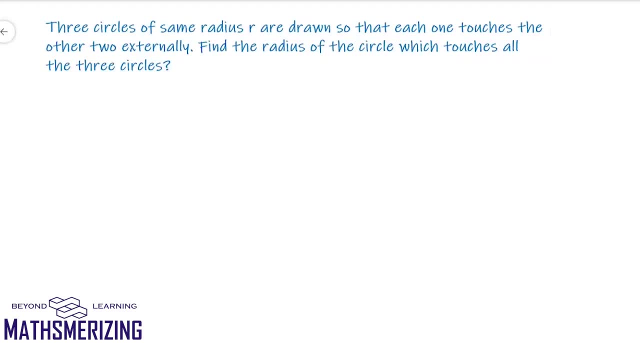 can still use Descartes theorem of kissing circles. Let us take up an example Now. the question says there are three circles of same radius, r, and they touch each other externally. We have to find the radius of a circle which touches all the three circles. So I am given three circles. 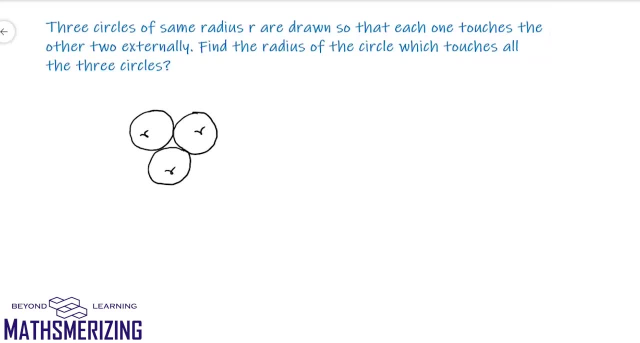 and they are the same radius r, and they touch each other externally. Now we have to find the radius of the circle which touches all the three circles. So there can be a circle which externally touches all the three circles and there can be a circle which touches all the three circles internally also. 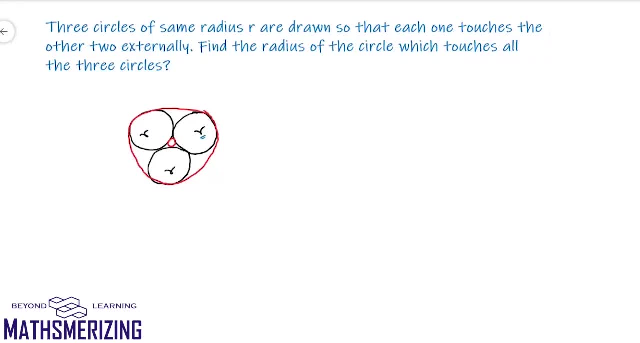 Now, because all the three circles, they touch each other externally. here the curvature can be defined as: k1 equals k2 equals k3, and that is equal to plus one upon two. Now Descartes theorem states that k4 is equal to k1 plus k2, plus k3 plus minus twice under root of. 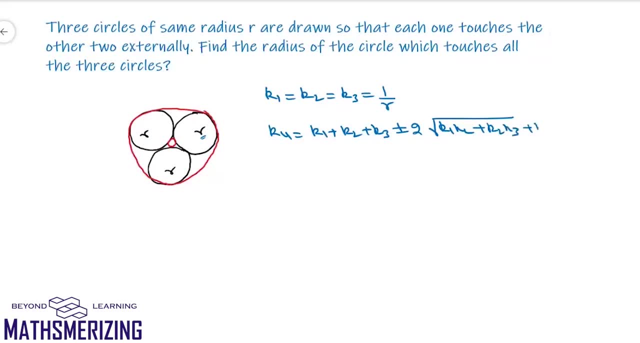 k1, k2 plus k2, k3 plus k3, k1.. So if I will put the value of k1, k2 and k3, I will get k4 as 3 upon r plus minus twice under root of r, 3 upon R, square. so I can write as 3 plus or minus twice under root 3 upon R. Now if I 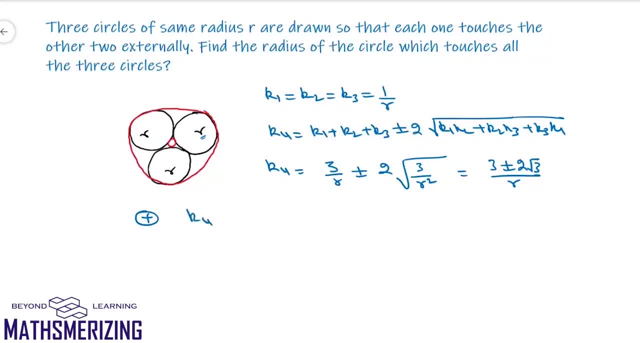 take plus sign, I will get K4 as 3 plus 2 root 3 upon R. Now if I take the reciprocal I can find the radius of the fourth circle. so in that case R4 will be given by R upon 3 plus 2 root 3. and if I take root 3 common, I can write it as root 3 and this is 2 plus root. 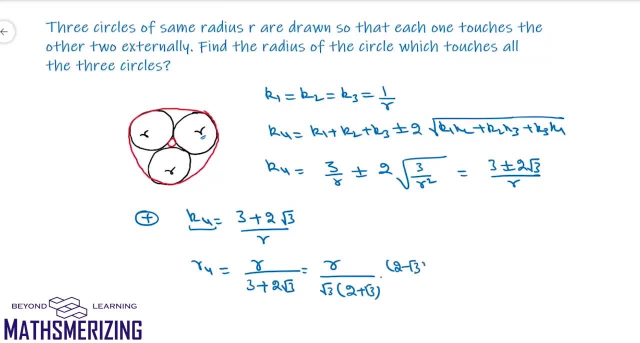 3 and if I rationalize, I can write it as 2 minus root, 3, R upon under root, 3 upon R. So in this case it will represent radius of the circle which touches the given circles externally. that is the radius of this smaller circle. Now we will take minus sign in that case. I. 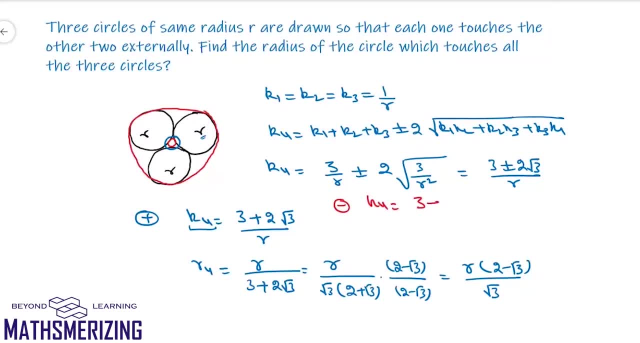 will get this K4 as 3 minus 2 root 3 upon R. Now in this case this curvature is negative, so it represents that this circle it is going to touch the given circles internally. So if I have to find radius so I can write R4 as R upon and I need to change the sign because radius has to be positive. 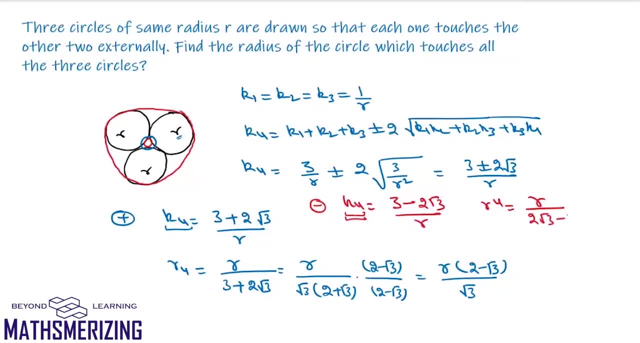 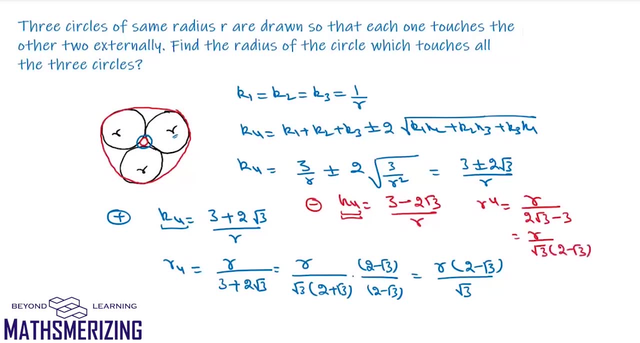 so I can write it as twice root 3 minus 3. so again I will take root 3 common. so this is 2 minus root 3. again I will rationalize. so in that case the value of R4 is 2 minus root 3.. 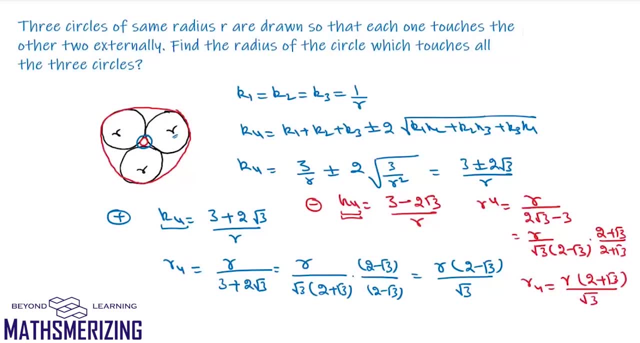 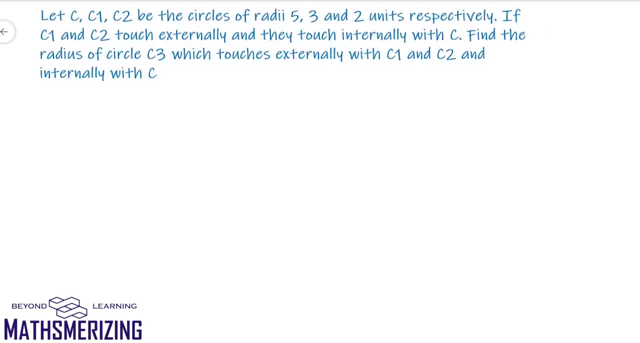 R into 2 plus root 3 by root 3 and in this case this R4, it represents radius of the larger circle. Now in this question it says there are three circles: C, C1 and C2, and their radiuses are 5, 3 and 2 respectively if C1 and C2 touch externally. so we have two circles which touch 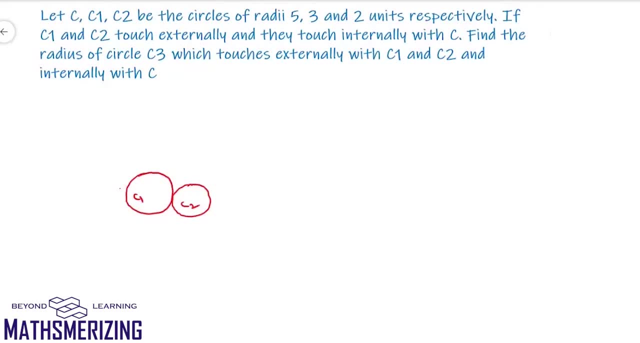 each other externally. And then there is another circle, C, which touches the given circles internally. So we have three circles that touch each other. Now there is another circle, C3, which touches C1 and C2 externally and C internally. So there is another circle which touches C internally and C1 and C2 externally. 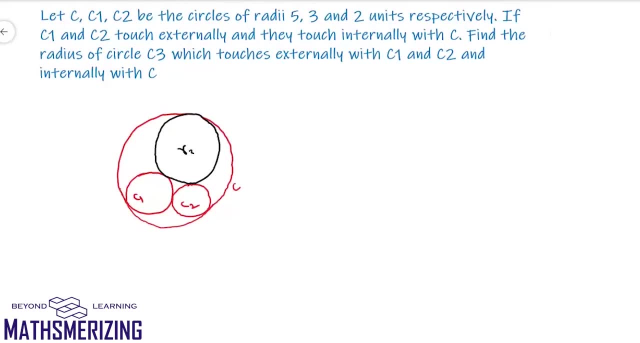 externally. we have to find the radius of this third circle. Now we know that in this case, K1 will be positive, So it will be 1 upon R1, which is 1 by 3.. K2 will be positive, So it will be 1 by R2 and there will be 1 by 2, because they touch each other externally. 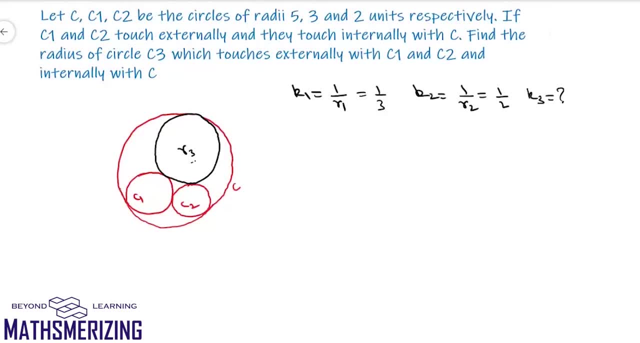 Now K3,. K3 is the curvature of the circle that we have to find, And suppose I'll say curvature of this outer circle is K4, and because the circle touches them internally, so it will be negative, So it will be minus 1 upon R, So there'll be minus 1 by 5.. Now if we 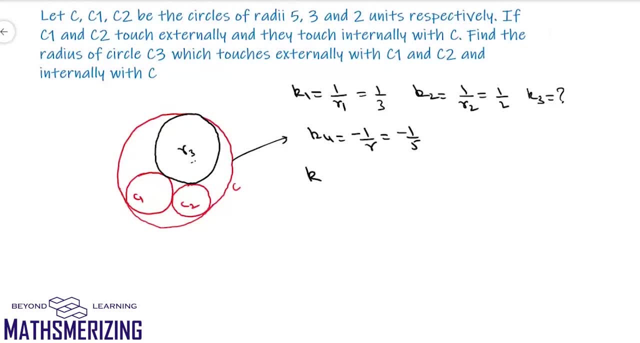 use Descartes theorem, I can write K3 as K3 equals K1 plus K2 plus K4 plus minus, twice under root. Okay, Okay, Okay, Okay. K1, K2, K2, K4, K4, K1.. So now I'll put the value of K1, K2 and K4. So I'll get K3 as 1. 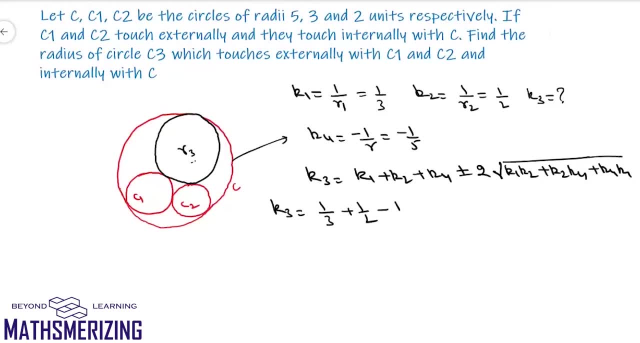 upon 3 plus 1 upon 2 minus 1 upon 5 plus minus twice. under root This is 1 by 6 minus 1 by 15.. So if I'll take LCM 30. So this is 10 plus 15 minus 6 and this is plus minus twice. 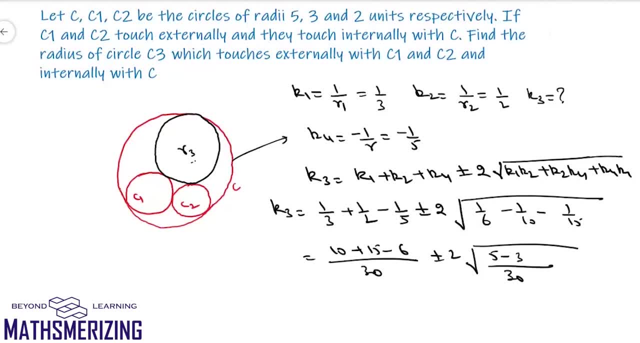 And here again it will be 30,, 5,, 3 and 2.. So I'll get K3 as 25 minus 6 is 19 by 30 and plus minus 0. So from here I can say the value of R2 is 0. So I'll get K3 as 25 minus 6 is. 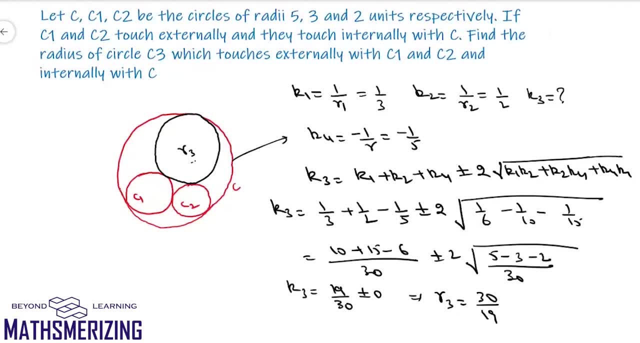 0. So from here I can say the value of R3 is 30 by 19.. So there is only one circle possible in this case, and the radius of that circle is given by 30 by 19 units. Now let us consider: 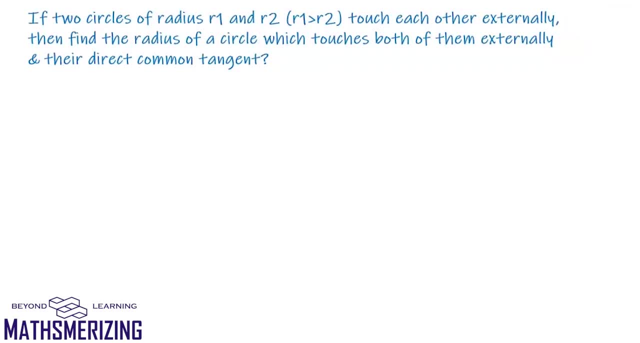 the case of a degenerate circle. So in this case we have two circles of radius, R1 and R2, and R1 is greater than R2.. Now we have to find the radius of a circle which touches both the circle externally and also their 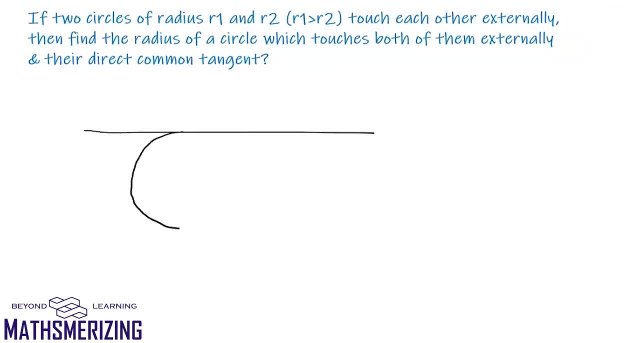 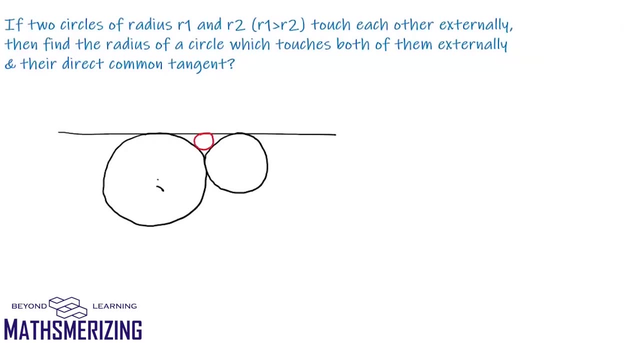 direct common tangent. So in this case we have two circles. The radius of first circle is R1 and the radius of second circle is R2.. Now we don't have a third circle, but we have a straight line and we know that straight line is a degenerate circle. So in this case, 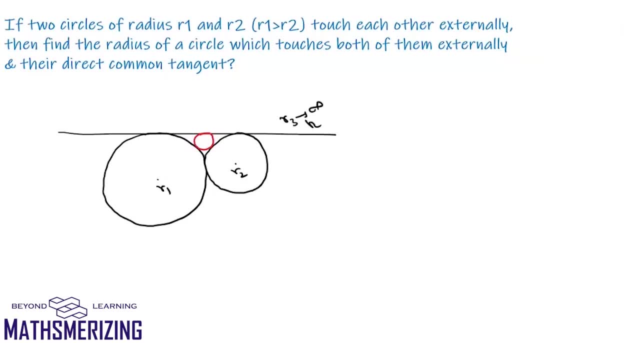 R3 will be infinite and K3 will be 0 and we have to find the radius of the smaller circle. Now we use Descartes theorem. We can write: k equals k1 plus k2 plus k3 plus minus, twice under root. 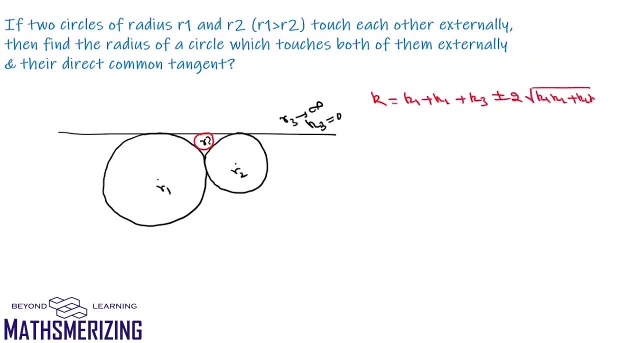 k1, k2 plus k2, k3 plus k3, k1.Now k1 is 1 upon R2, again will be positive, and k2 is 1 upon R2, again will be positive, nk3. else then K3 is 0. so I can write K as 1 upon R1 plus 1 upon R2, plus 0 and plus minus twice. 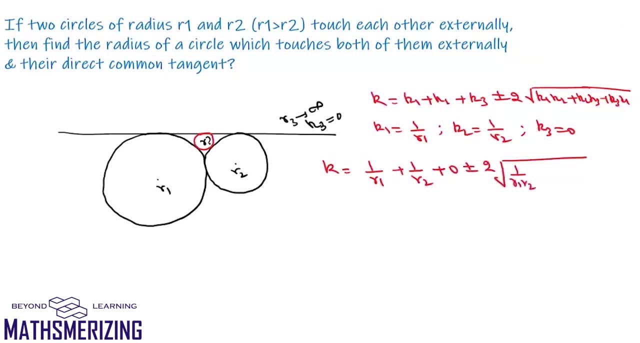 under root of 1 upon R1- R2 and plus 0 plus 0. so if I take LCM I can write it as R1- R2 and this R2 plus R1 plus minus twice under root R1- R2, so I can write K as under root. 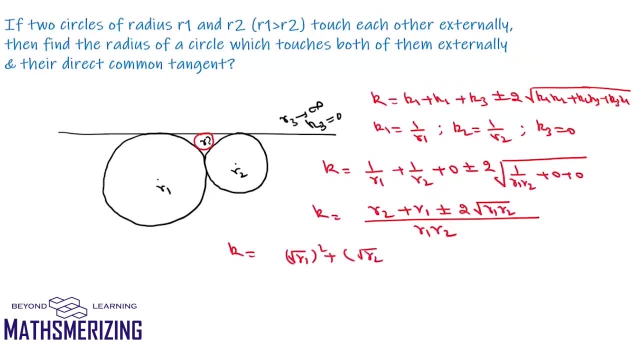 of R1 square plus under root of R2, square plus minus twice under root of R1 R2 upon R1 R2, so I can write it as under root of R1 plus minus under root of R2.. it is 2, somewhat similar.